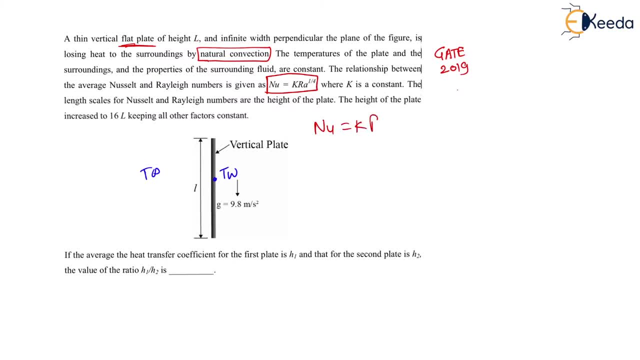 That is, Nusselt number is equal to K into Relake number power 1 by 2.. Now where K is constant, Means they have given the relationship that Nusselt number is directly proportional to Relake number power 1 by 4.. 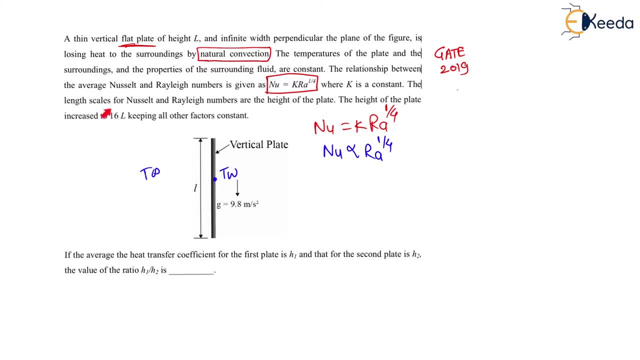 Then the length scale of the Nusselt and Relake number are the height of plate Means. here we have to consider this height of plate as a length characteristic dimension. Therefore here we can say that characteristic dimension is equal to L. Then the height of the plate increased to 2.. 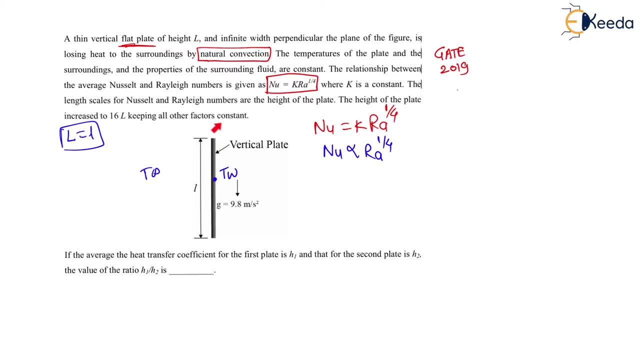 Plate increased to 16 L, keeping all other factors constants. Now here, my dear students. this height of plate is increased 16 times Means here the L2 is becoming L2 is equal to 16 times L1.. Now that means the height is increased by 16 times. 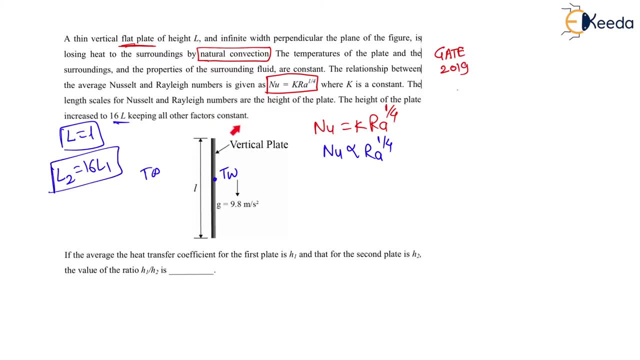 Then keeping all other factors constant Means there is no change in any other parameter except length. Then If the average heat transfer coefficient for the first plate is H1. And that of for the second plate is H2., Then the value of ratio of H1 divided by H2 is: 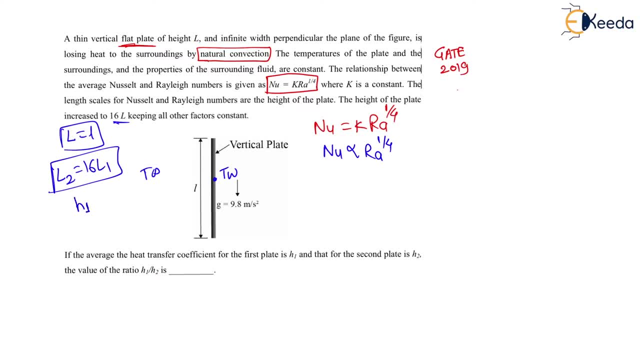 Then we have to find average heat transfer coefficient in first case divided by average heat transfer coefficient in second case. So, my dear students, in this question they are asking relation between average heat transfer coefficients And they have given relation between lengths, Means here, with respect to change in length. 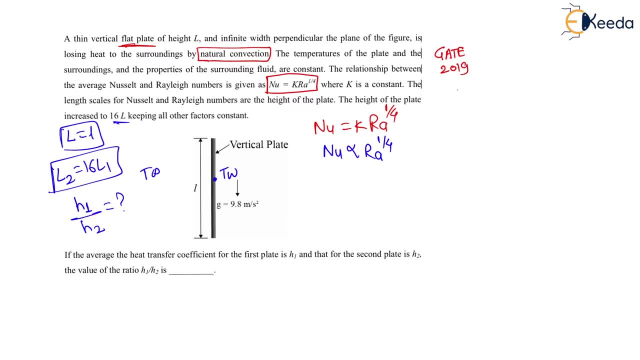 Only the average heat transfer coefficient, H, is changing, And all other parameters we have to consider constant, Right? Therefore, here there is a variation in H and length. Now, my dear students, we know that this Nusselt number is nothing but HL divided by K. 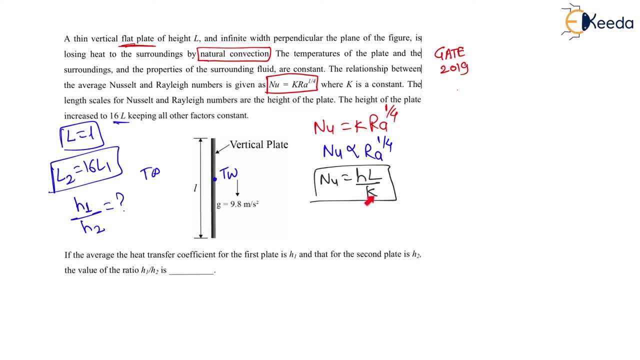 Right, That formula we have seen. this Nusselt number is nothing but HL divided by K. Therefore, can I say: this Nusselt number is directly proportional to H and L. Therefore we can say: the Nusselt number is directly proportional to H and L. 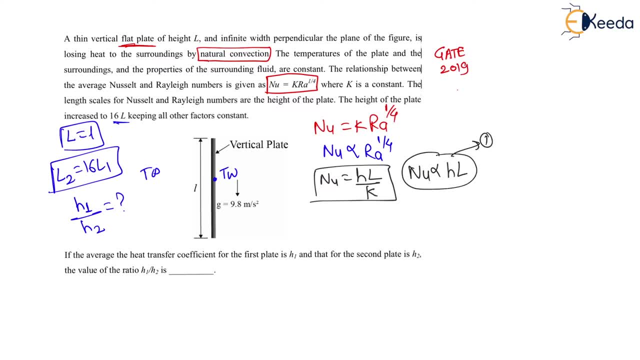 This is important relation, Relation number one. And my dear students here, This relay number, Nusselt number, is directly proportional to relay number power 1 by 4.. Right, So again we have one more relation: Nusselt number is directly proportional to relay number power 1 by 4.. 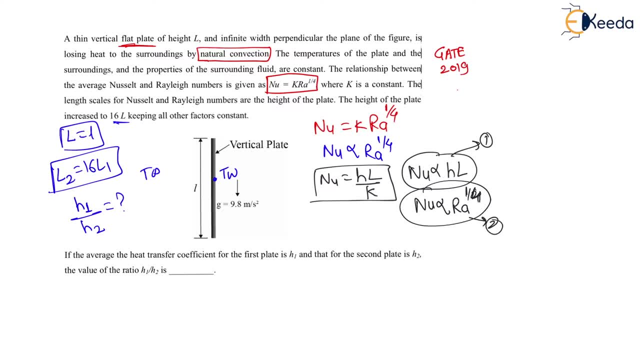 1 by 4.. Right, This is the second relation. Now, my dear students, this relay number is nothing but product of Grashof number and frontal number That already we have defined in numbers used in convection. That relay number is product of Grashof number and frontal number. 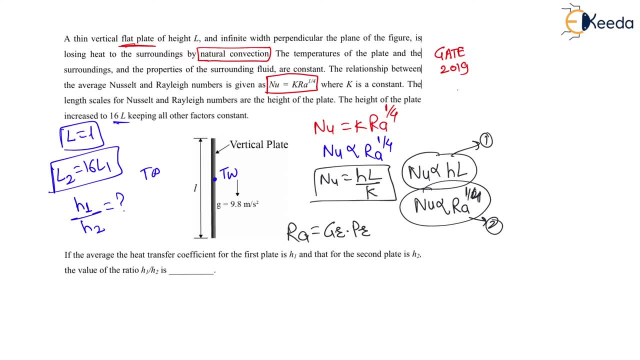 Right, And we must know that. what is the formula of Grashof number? Now, my dear students, the Grashof number is nothing but rho, square L, cube G, beta, delta T, divided by mu, square Right, Where rho is the density of fluid. 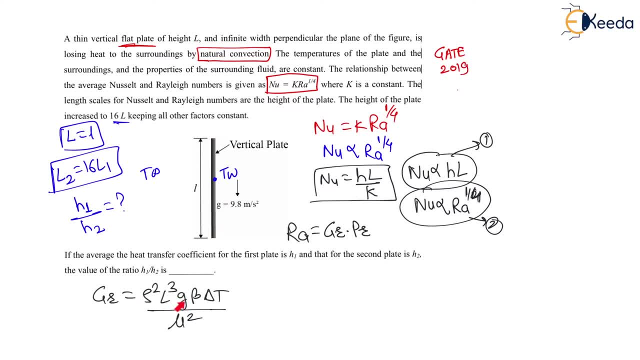 L is the characteristic dimension here, G is the acceleration due to gravity, Beta is isomeric volume expansion coefficient. Delta T is temperature change, That is wall temperature minus surrounding temperature T, infinity. And mu is here dynamic viscosity. Right, Mu is the dynamic viscosity. 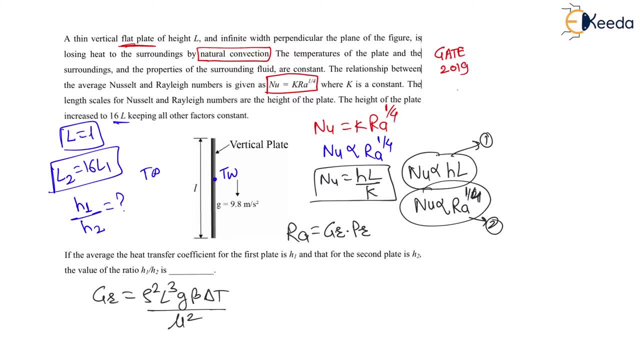 Right Now, my dear students, after this Grashof number, Let us understand this frontal number. Frontal number is nothing but mu, Cp divided by K, Where mu is nothing but dynamic viscosity, Cp is specific heat at constant pressure and K is the thermal conductivity of that fluid. 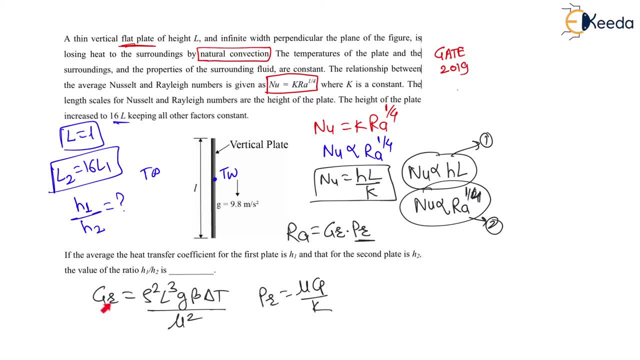 Right, These are the two numbers. Now, my dear students, Here we know the formula of Grashof number, We know the formula of frontal number. Therefore, can I say this: relay number Ra is equal to Grashof number, which is nothing but rho square, L, cube G, beta, delta T divided by mu square. 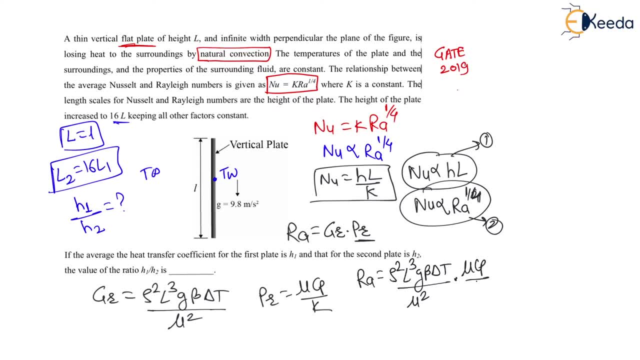 Into frontal number, which is nothing but mu Cp divided by K Right. This should be our relay number. And my dear students here they are mentioning that only H and L is changing. All other factors are constant Means. can I say here: this relay number is directly proportional to L cube. 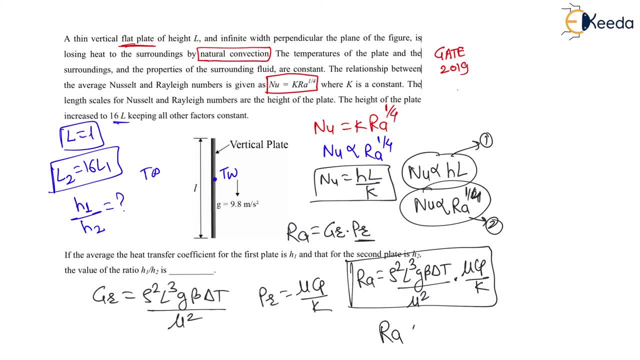 Right. Therefore, we got one more relation: Relay number is directly proportional to L cube, Because here only length of plate is changing. All other parameters are constant, Right. So, my dear students, very important relation we got, So let us write down this. important relations. 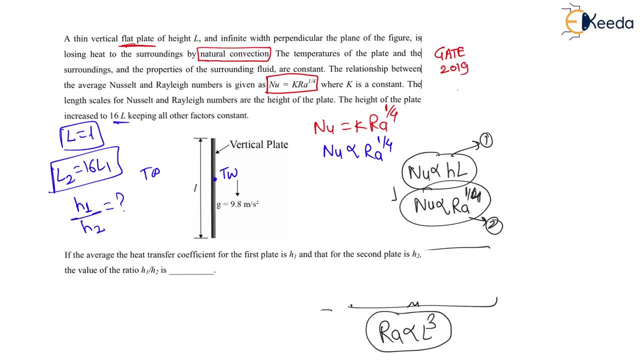 Right. So here this is our third relation, That is, relay number is directly proportional to L cube. Therefore, relay number is directly proportional to L cube. Let us say this is the third relation. Now, my dear students, with the help of relation 1, relation 2 and relation 3.. 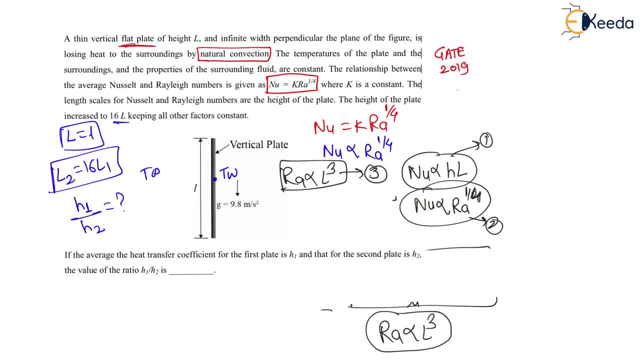 Let us define the relation between H and L Right Now. let us define them Now. it is very simple. now Everything is understood. Now, here we have to put the values and we have to derive for the relationship Right Now, here, very first relation is Nusselt. number is directly proportional to H- L. 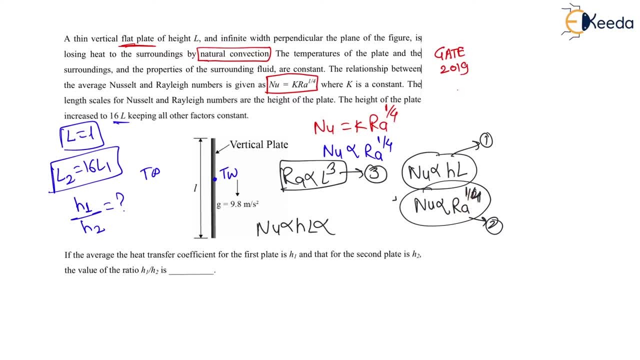 And again this second relation: Nusselt number is directly proportional to relay number power 1 by 4.. It is directly proportional to relay number power 1 by 4.. But, my dear students, relay number is directly proportional to L cube. Therefore, can I say this Nusselt number is directly proportional to H L? 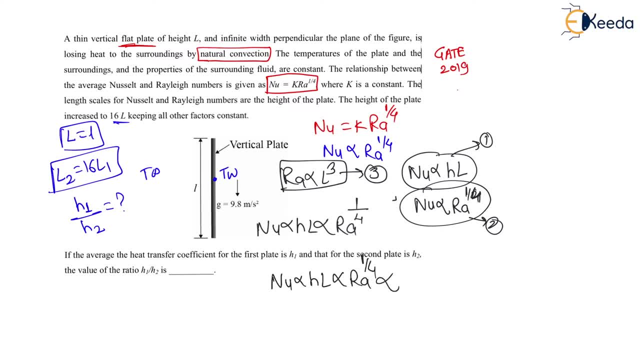 Which is directly proportional to relay number power 1 by 4.. Is directly proportional to relay number, is directly proportional to L cube, But it is relay number power 1 by 4.. Therefore, it will become L cube power 1 by 4.. 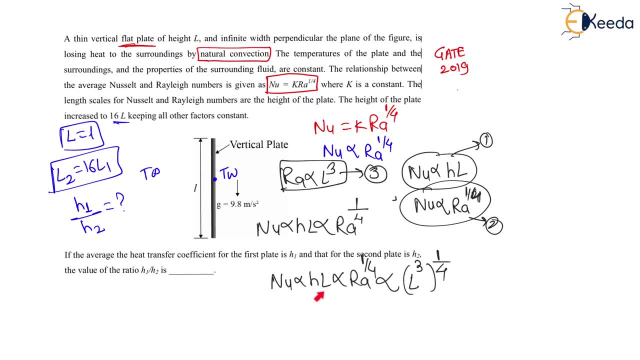 Right? This will be our final relation. Therefore, my dear students, here H is required and L is given. So let us equate these two terms, Right? So in this final relationship, we have to consider H, L term only, Right? So, my dear students, what will be the now result? 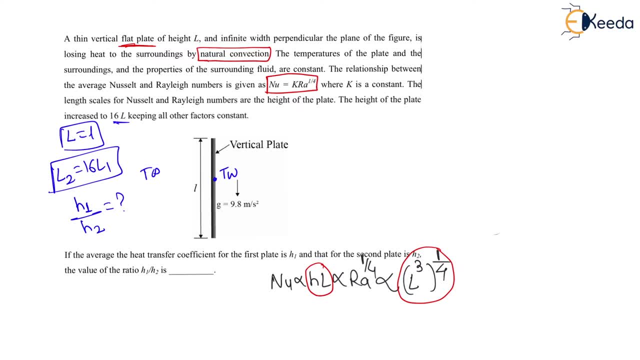 Let us find the result now. Now, everything is now known here. Right Now, let us equate them. Therefore, I can say here this: H: L is directly proportional to L power 1 by 4.. L power: 3 by 4.. 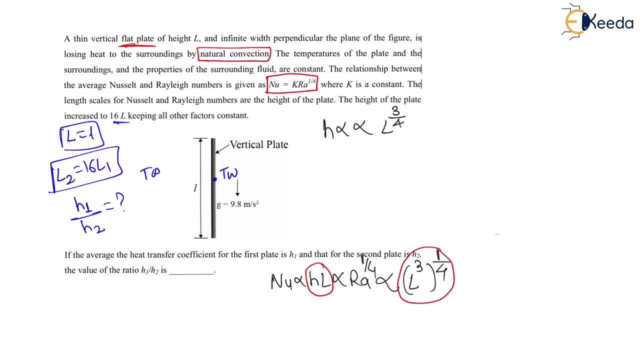 Right, H? L is directly proportional to- Wait Sorry, Just a minute Here. H? L is directly proportional to L power 3 by 4.. Therefore can I say here this: H will be directly proportional to L power 3 by 4 divided by L. 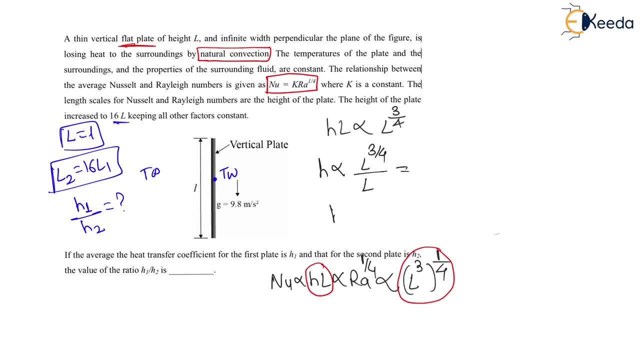 Therefore, it will become: H is directly proportional to L power 3 by 4 minus 1.. Which will be equal to Right. Therefore, let us find this relationship. Therefore, again, H is directly proportional to L power 3 minus 4 divided by 4.. 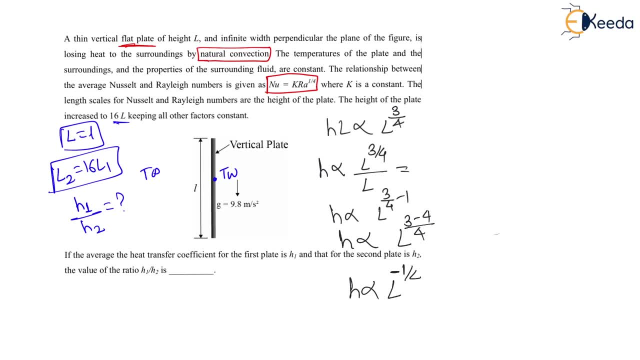 Therefore, H is directly proportional to L power minus 1 by 4.. This will be our final relation between H and L And, my dear students, here length is increasing by 16 times. So what will be H1 divided by H2.. Now if I want to consider relation that is, H1 divided by H2..